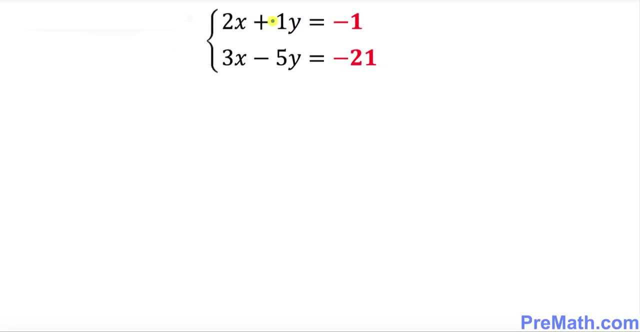 later on and over here, make sure if there's any coefficient is missing, put down like y was there, so I put down one times Y. So now let's go ahead and and get started. okay, so we want to solve this system means that we are looking for. 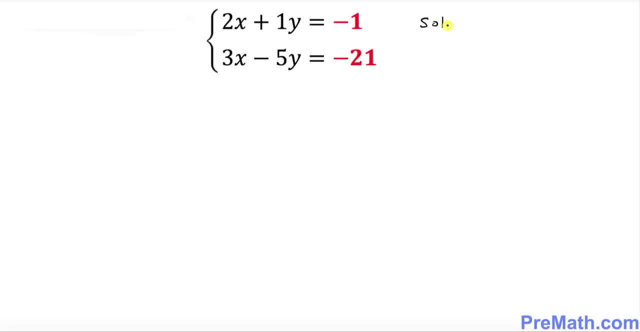 unknown variables. what are our variables that we are looking for? we want to solve? this thing means we want to solve for x and y, isn't it? that means we are looking for x value and we are looking for y value. so here we're gonna play a small kind of game. okay, go ahead, let's get started. i want you. 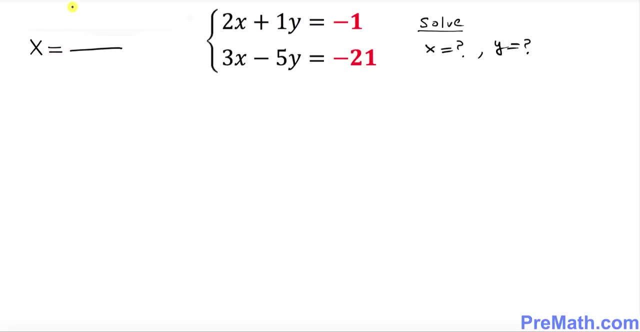 to put down x right up here. i want you to put one box on the top and one box on the bottom. likewise, i want you to put for y same thing: put one box on the bottom, on the top, and one on the bottom. and, by the way, these boxes are called determinants, are simply determinant, just keep. 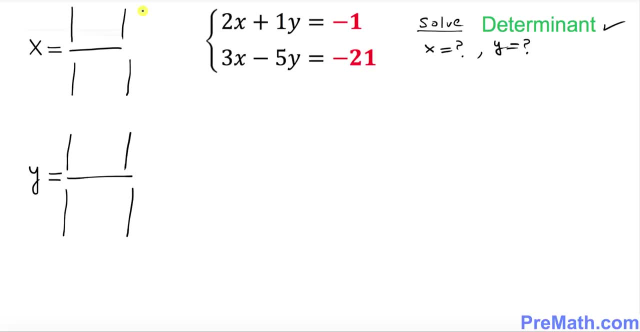 in your mind. they have a special name: determinant. now, next step. i want you to just go see over here. i, we want to fill out these determinants. are these boxes? look at these coefficients on the left hand side: two, one, three and negative five. whatever these numbers are, i. 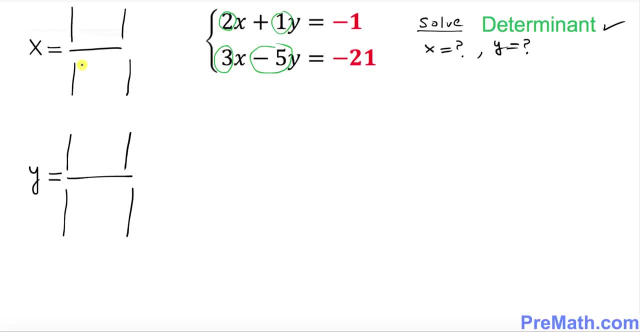 want you to put in the bottom determinants in the same order. so you're going to have two, one, three negative five, same numbers on the the next bottom: same thing, same numbers: two, one, three negative five. so far, so good. the next thing: i want you to look at these red numbers in the red. i want you 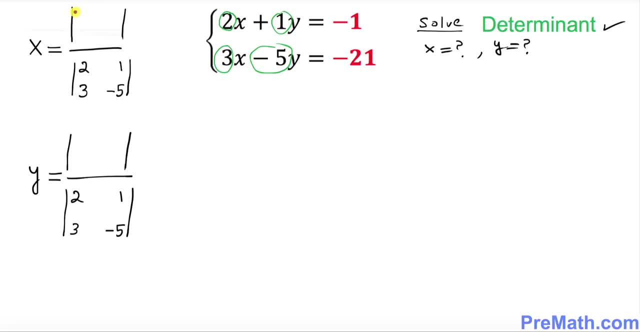 to put in in the first, for x is going to be first column, so negative one and negative 21, and for y it shifts to the negative. uh, the next column, negative one and negative 21. so far, so good. now we need to fill out this second column. 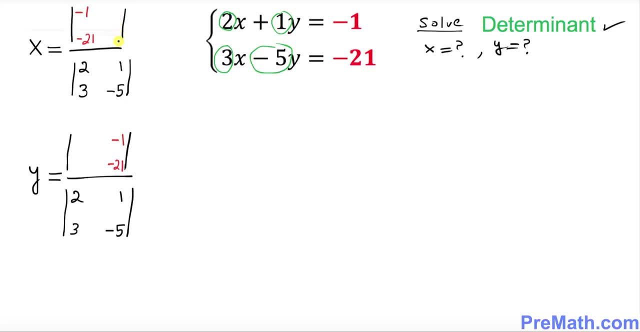 look at the numbers right underneath this column. what are the numbers below this empty column? this is one negative five. i want you to push these numbers up, copy and paste, so those going to be same number: one negative five. and likewise over here for this empty column to be filled out. look at the numbers below, which is two and three. push them up or simply. 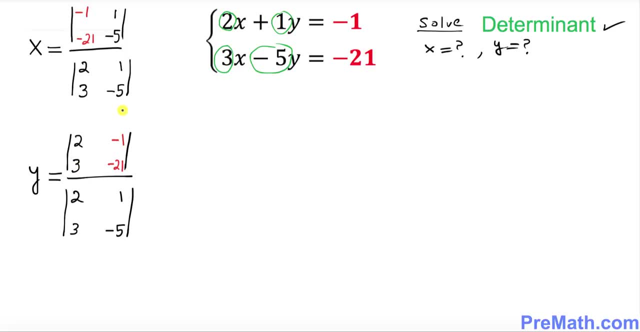 copy and paste, this become two and three. so we have nicely set up these x and y, these boxes. now we're gonna find the value of these determinants. and here i have put down this top determinant right up here. i'm gonna find the value or evaluate it. 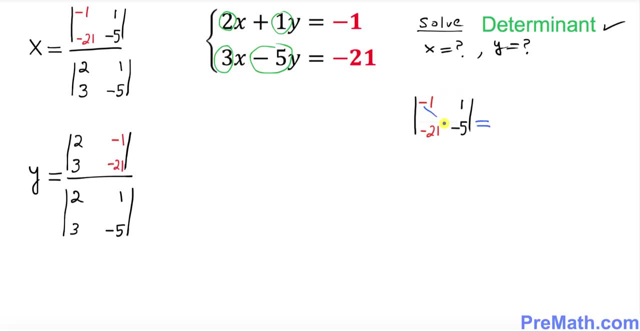 so let me show you really super easy method. i want you to cross multiply this way: all right, negative one times negative five is gonna be positive five, and after that one always, always put down a minus sign. okay. and then i want you to cross multiply the other way around. so one times negative, 21. 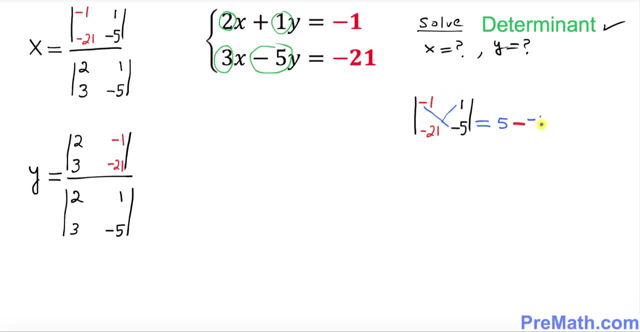 equals to negative 21. do you see that one? now, when you have a two negative each other, they become positive. so we got 5 plus 21, equal to 26. so the value of this top determinant? this value turns out to be 26. all right, so far, so good. and now we're going to find the value of this bottom determinant. 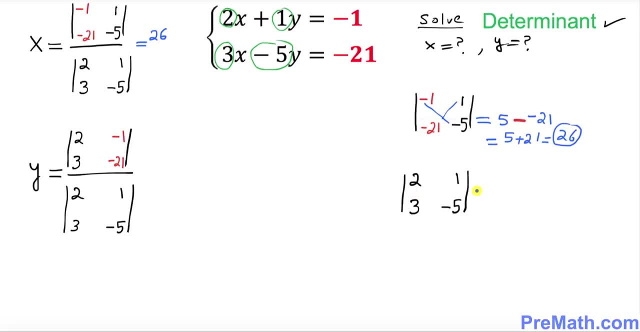 and now here is the bottom determinant, as you can see. let's go ahead and evaluate this one. we're going to do the same thing, same way we did before, exactly same way: 2 times negative. 5 is negative 10 and right after that one, i want you to put a minus. take away, sign minus and then i want 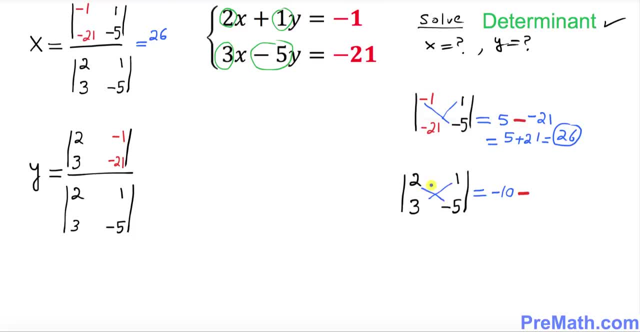 you to multiply the other cross, multiply the other way around. what we are doing is we are crisscrossing. so 1 times 3 is 3. that is going to give us negative 13.. so our the determinant of the bottom one turns out to be negative 13.. now you can see. the bottom determinants are same, so we don't have 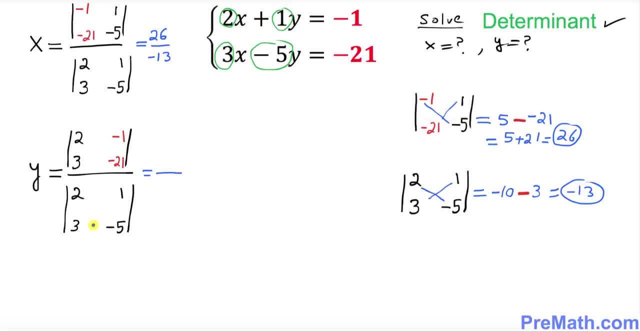 to do the bottom determinant all over again. we got the value, so this has a value negative 13 as well. and now we're going to find the value of this top determinant for y variable that. i put it down over here, copy it down and let's do exactly the way, same way as we did before crisscross. 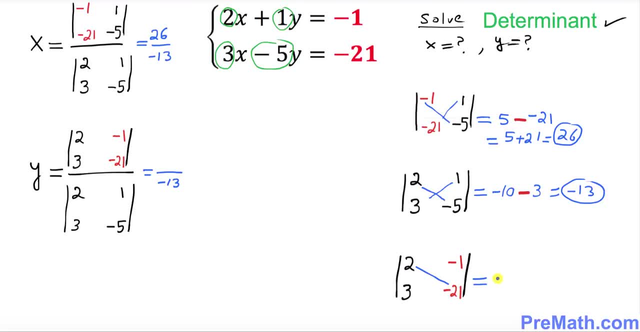 let's go first this way: 2 times negative 21 is negative 42. once again, as i told you before, i want you to put a minus our takeaway sign, and then the other way around. that is going to be negative 3, isn't it? so negative 3. so. 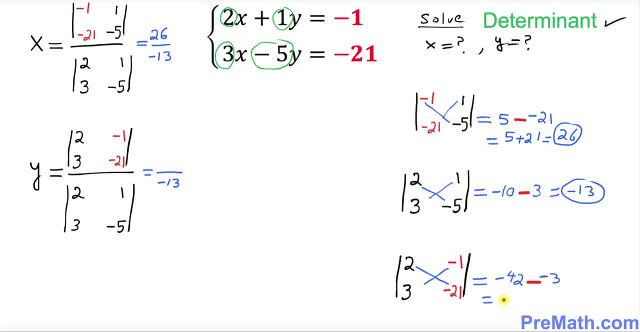 let's simplify that one so negative 42. negative and negative- they're next to each other- become positive plus 3. if you simplify that, becomes negative 39. so the value of this one turns out to be negative. 39. so if you simplify, reduce, this turns out to be simply negative. 2 over here and 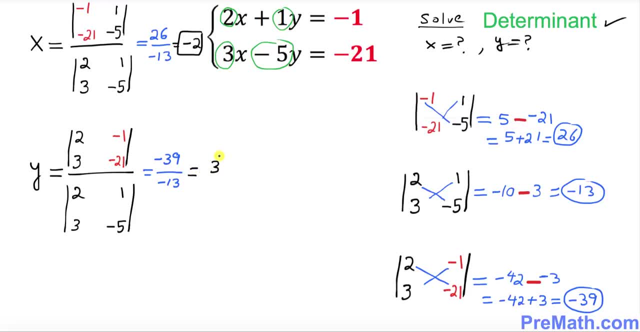 this turns out to be value of y is 3. thus, our solution turns out to be negative. 2 comma 3: 2 is your x value and 3 is your y value. Thanks for watching and please subscribe to my channel for more exciting videos.